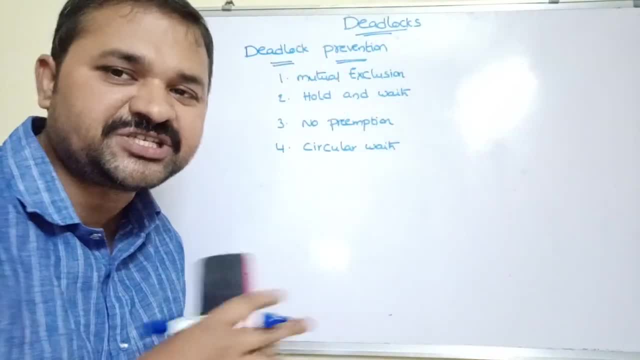 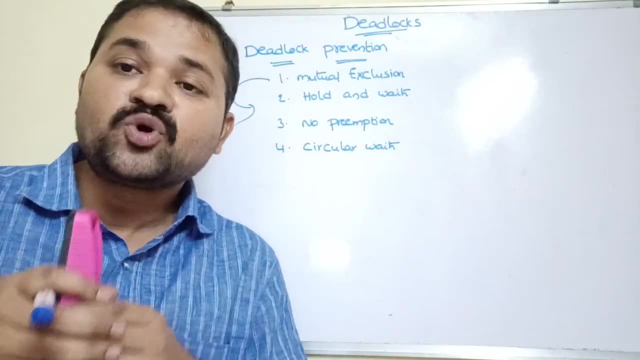 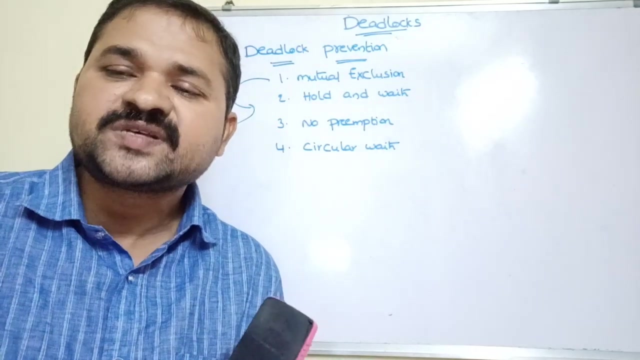 Let's check whether we can eliminate any one of these conditions or not. So what is the first one? Mutual extrusion. Mutual extrusion means a process can use only one resource at a time. That means all the resources are non shareable. by default, it is not possible to share a. 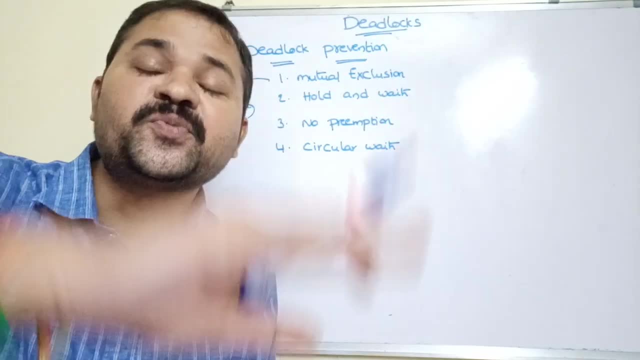 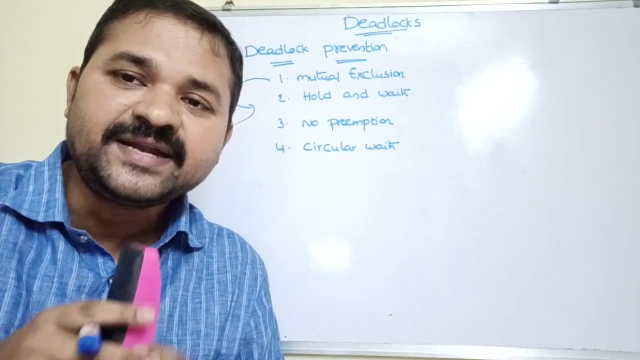 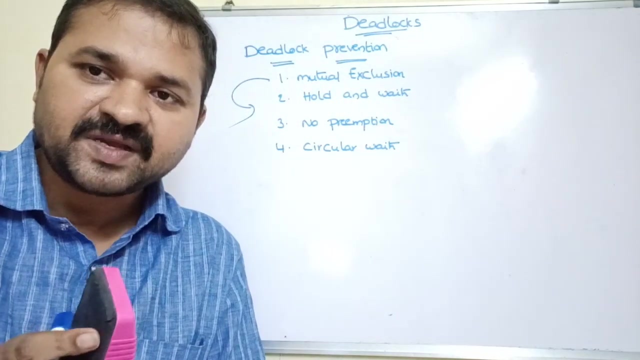 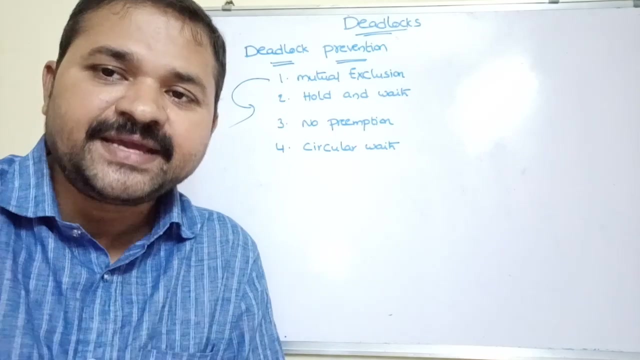 resource simultaneously among multiple processes. if we try to share a single resource among multiple processes simultaneously, then it will produces wrong results. let's take the example of a printer. let printer is shared between the process P1 and process P2 and if you perform printing then we will get the 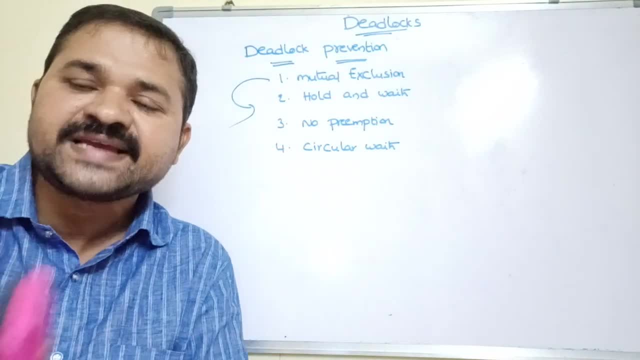 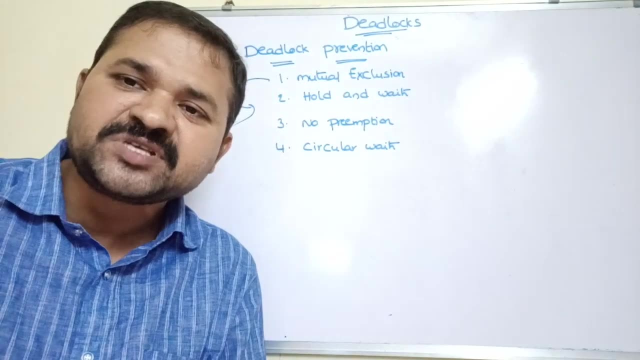 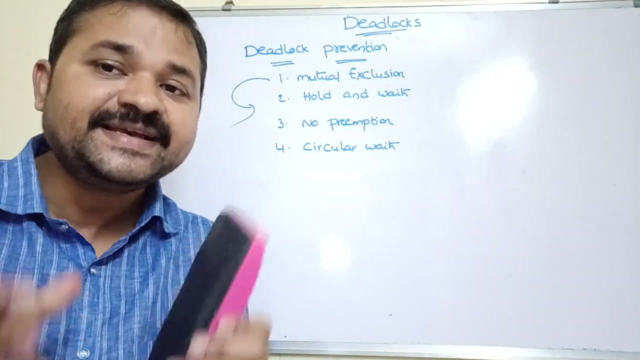 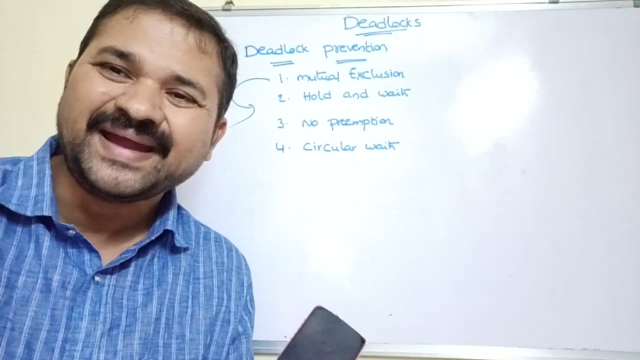 combination of P1 and P2 processes as the output. so that means it is producing wrong results. so it is not possible to eliminate mutual exclusion. so can we eliminate mutual exclusion? so it is not possible. it is not possible to eliminate mutual exclusion. why? because by default all the resources are non shareable if we share a single. 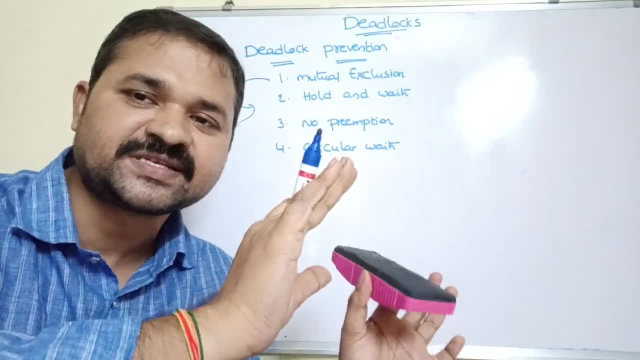 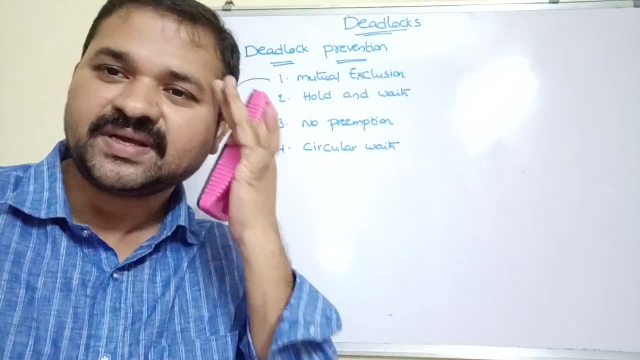 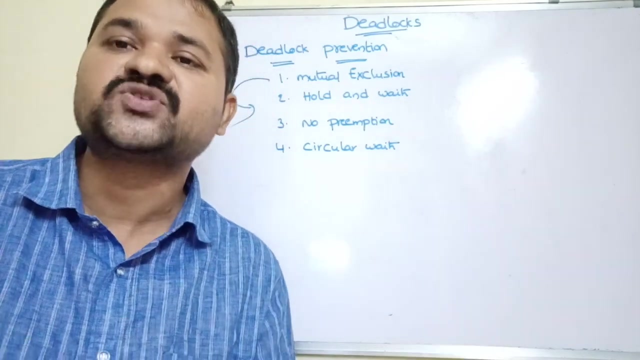 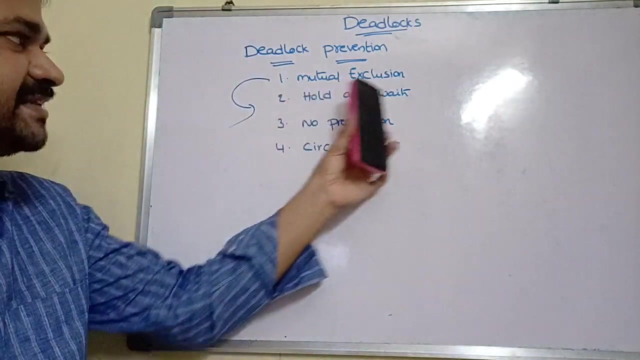 resource simultaneously among multiple processes, then we can say that mutual exclusion is eliminated. but that is not possible. it is not possible to share a resource simultaneously between multiple processes. so we can say that it is not possible to eliminate mutual exclusion. why? because by default all the resources are non shareable if we share a single. 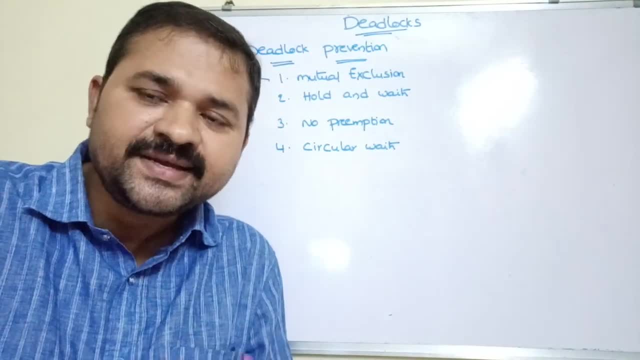 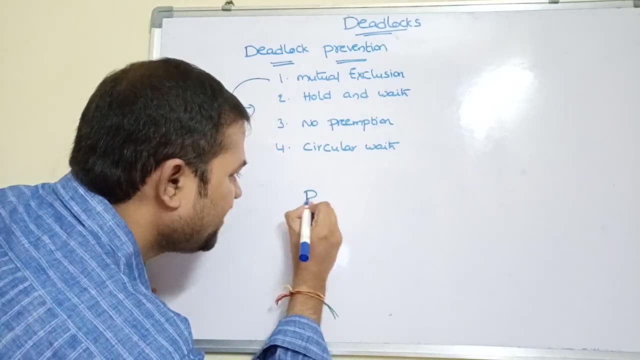 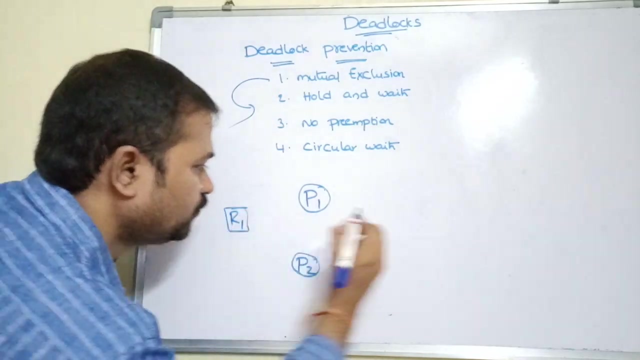 resource simultaneously between multiple processes, then we can say that it is not possible to eliminate mutual exclusion. lets see the next one. what is the next one? the next one: hold and wait. so we know what is hold and wait. a process is holding some resources and is waiting for other resources. 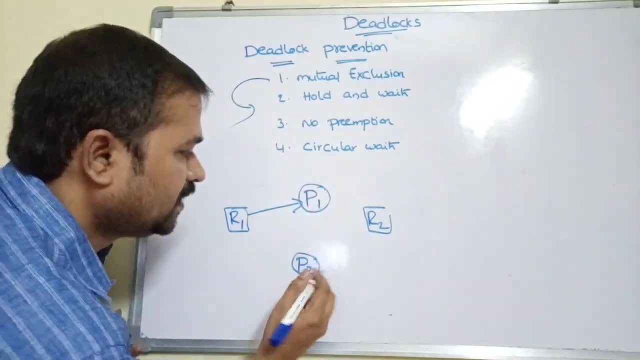 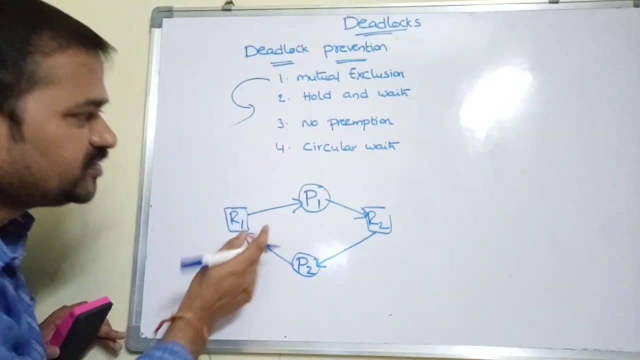 so we know what is hold and wait. a process is holding some resources- a and he's waiting R1, and P2 is holding R2.. P1 is waiting for R2.. P2 is waiting for R1.. So this situation is called. 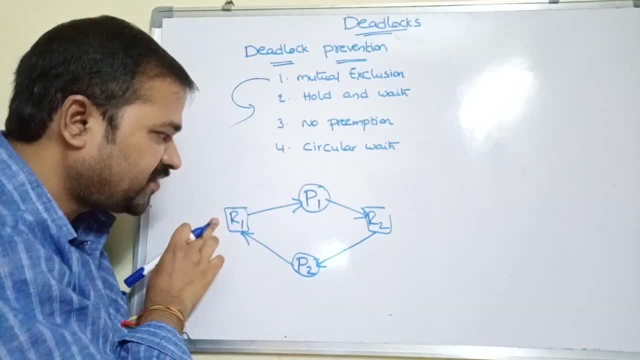 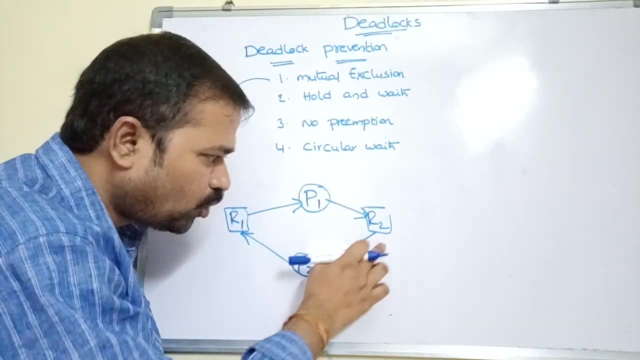 as hold and wait. Here P1 is holding R1 and is waiting for R2.. If we observe here about P2, P2 is holding R2 and it is waiting for R1.. So this situation is known as hold and wait. 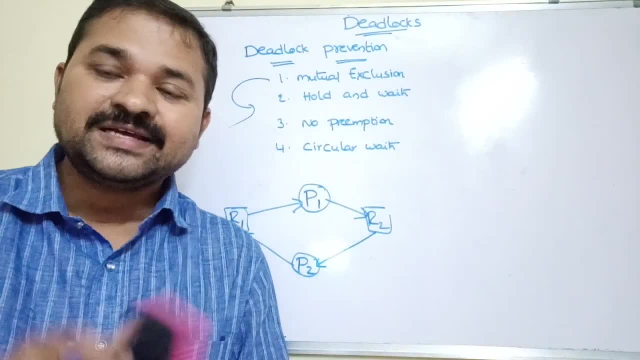 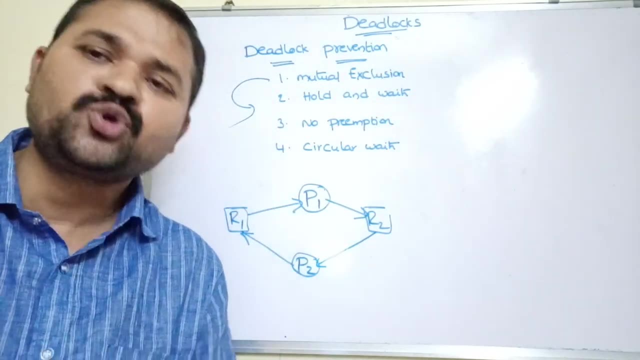 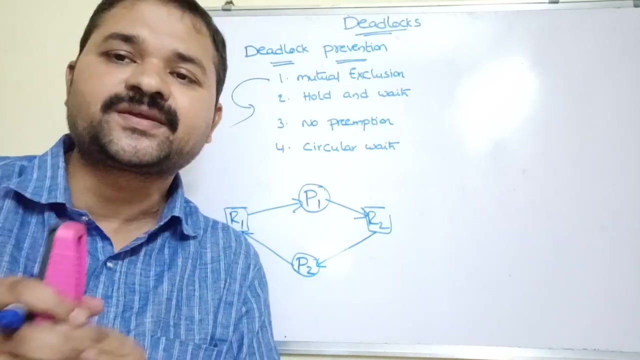 If hold and wait occurs in the system, then there is a possibility that deadlock may occur. Now let us check: Is it possible to eliminate hold and wait or not? There are two approaches in order to eliminate hold and wait. The first approach is a process can request for a resource. 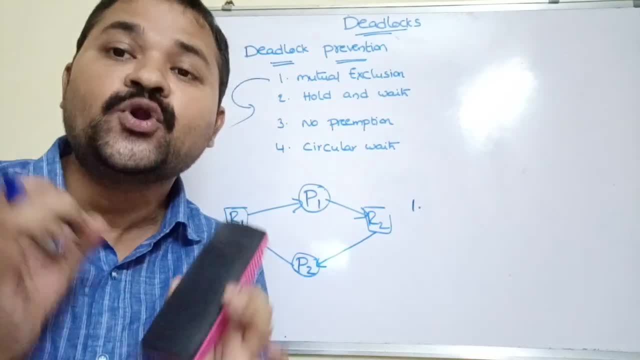 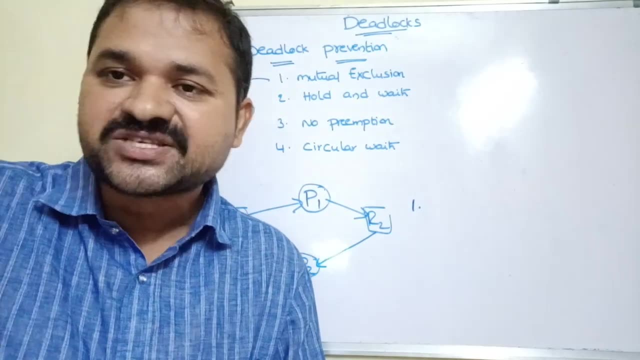 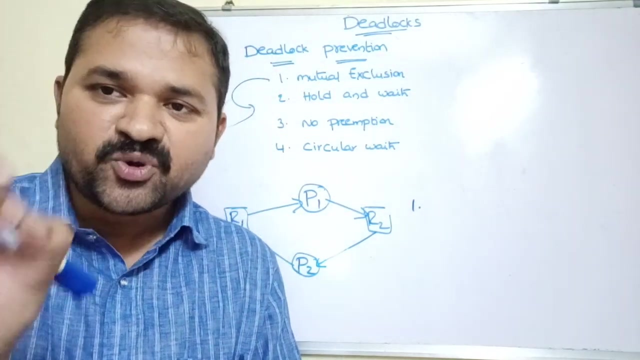 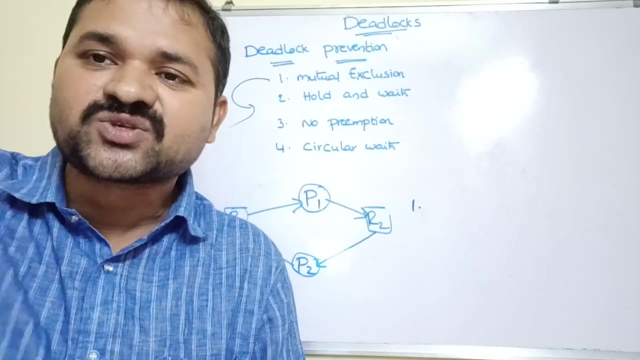 only when the process is holding no resources. So what is the first approach here? A process can request for a resource only when that process is holding no resources. So if the process does not hold any resources, then only that process has to put a request for other resources. So here there is only wait, is there? There is? 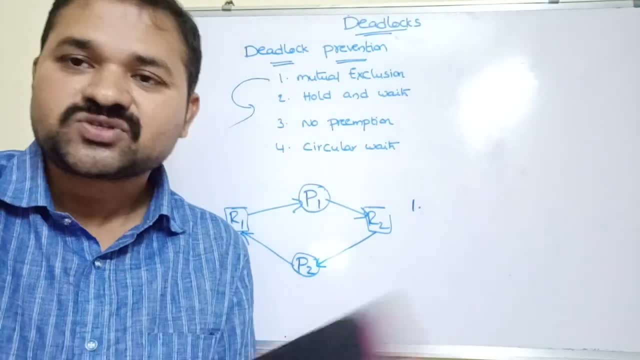 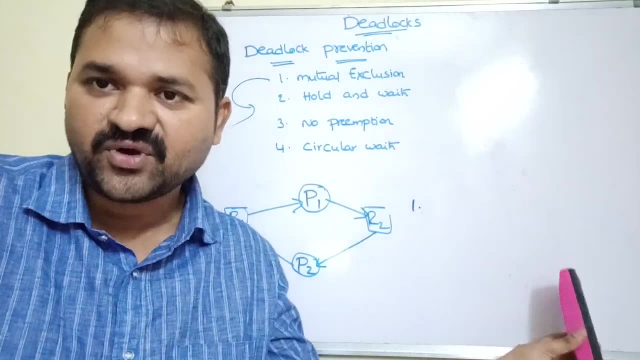 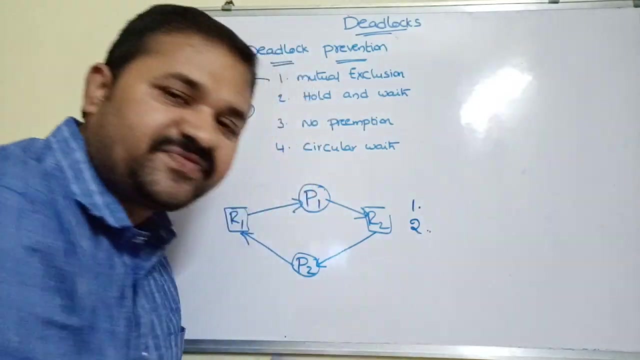 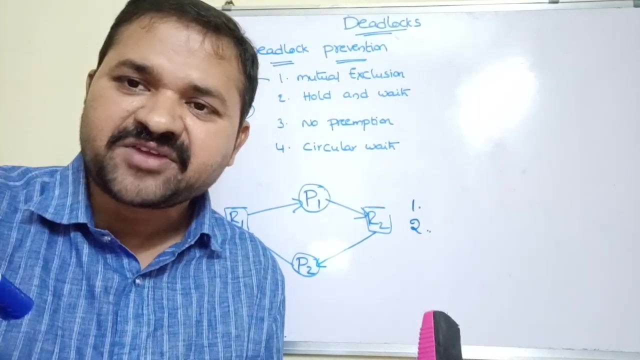 no hold here. There is no hold here, So that is why we can eliminate hold and wait. In this way, we can eliminate hold and wait. There is no hold situation here, Only wait situation. Let us see the second situation. First, the process has to put the request for all the resources. Let us assume that a process requires 5 resources in order to complete its execution. 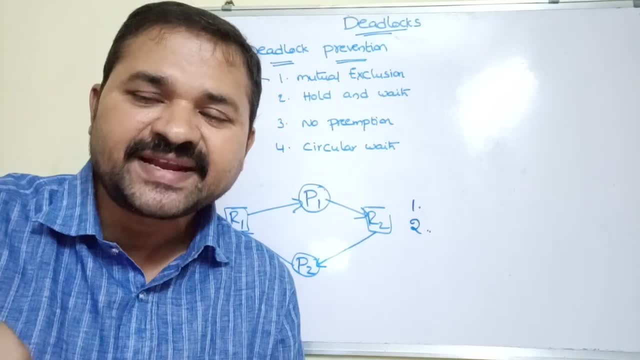 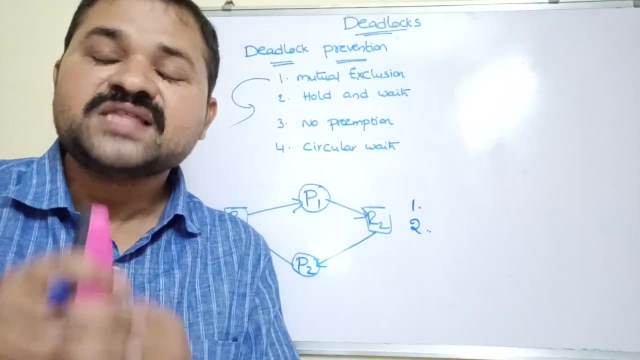 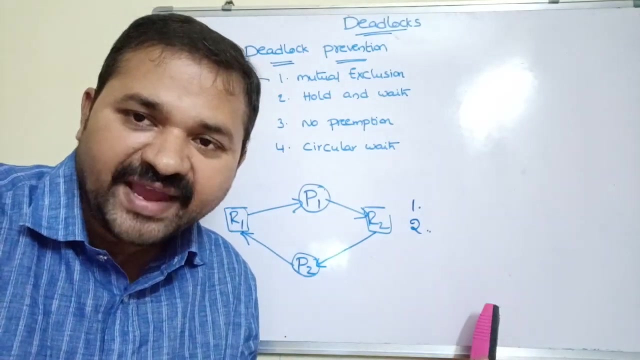 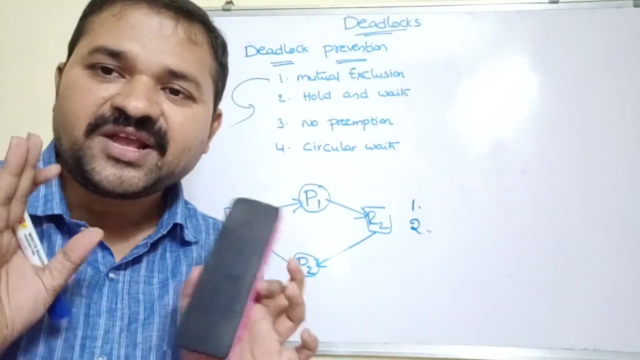 So first the corresponding process has to put the request for the 5 resources. So once the process has acquired the 5 resources, then only the process has to start the beginning of the execution. So here also there is no wait here, No hold and wait problem here: Once the process acquired all the resources, then only it has to start execution. 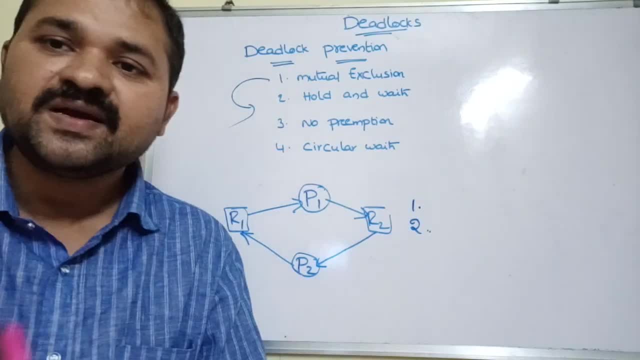 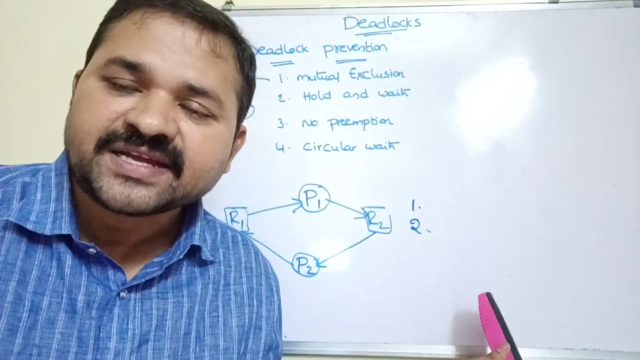 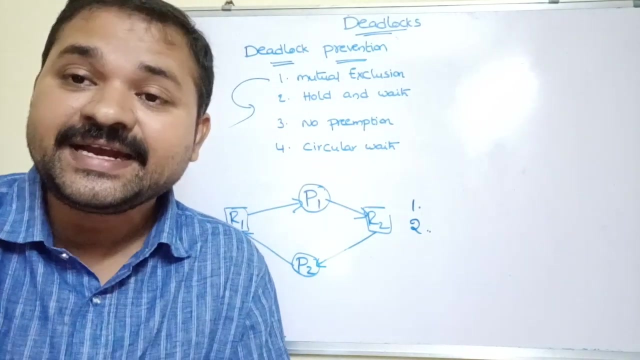 But the disadvantage of this approach also is that the process has to start the beginning of the execution. The first disadvantage is poor utilization of resources. Let us assume that the process has acquired 5 resources. One of the resources is printer. But when printer is needed, at the last page, only the printing is needed. 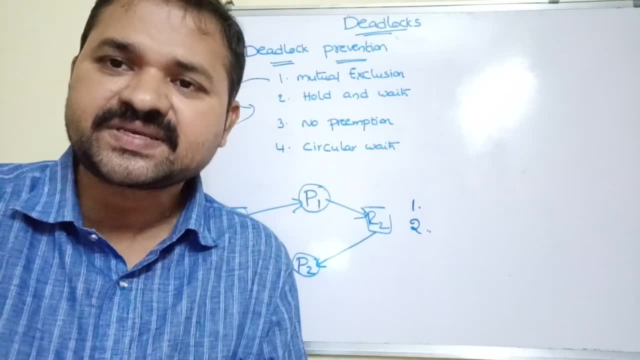 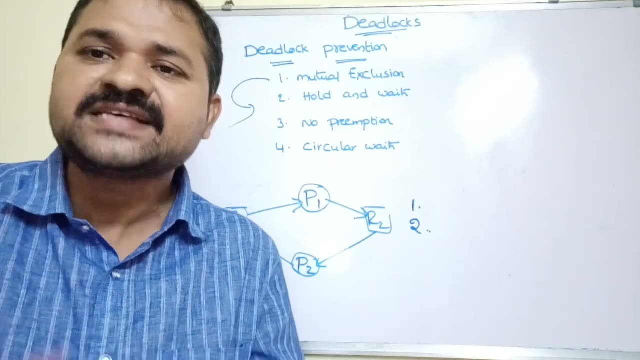 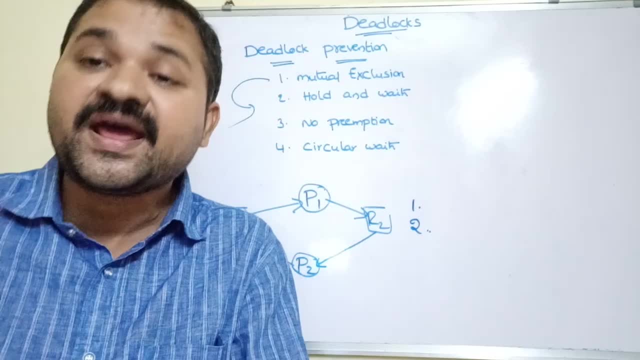 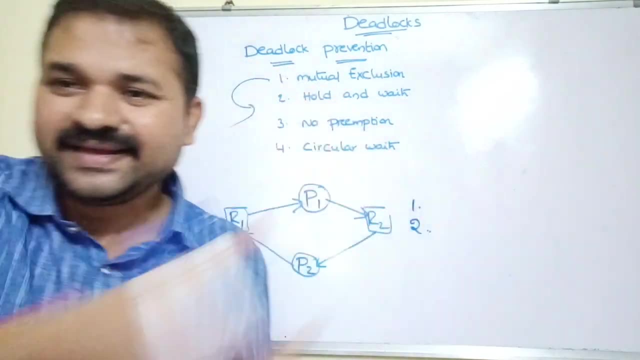 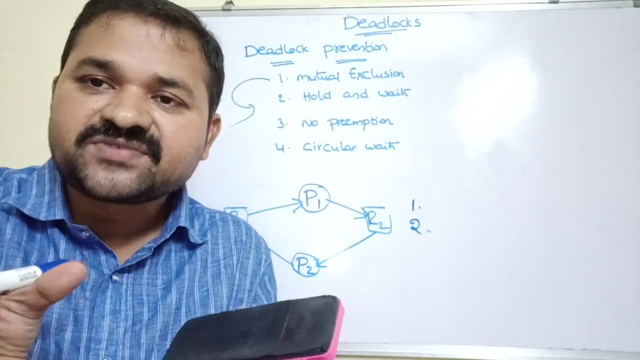 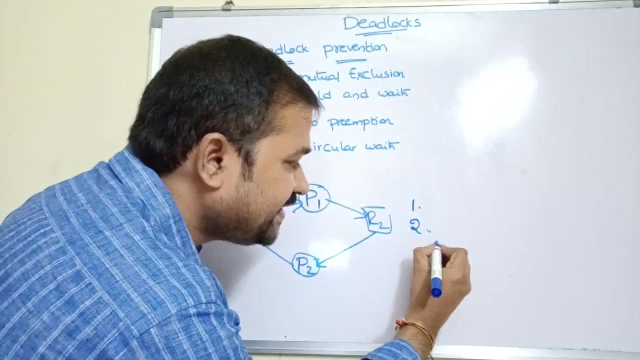 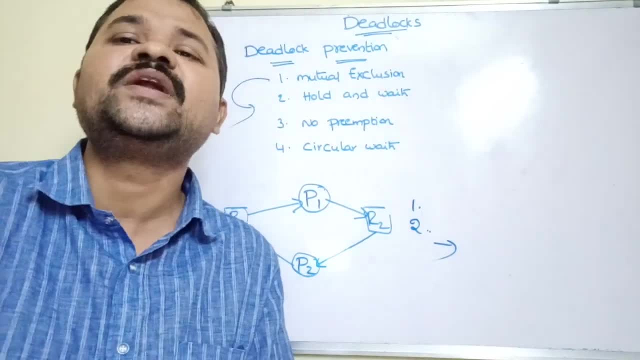 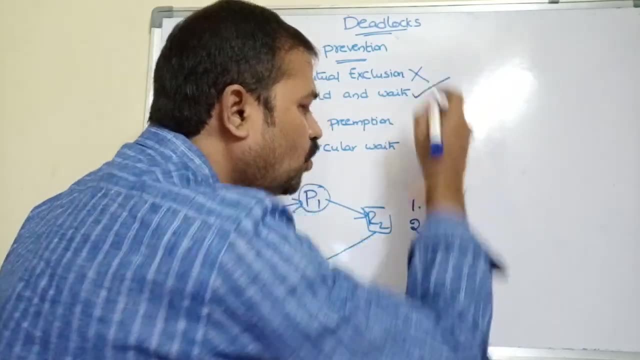 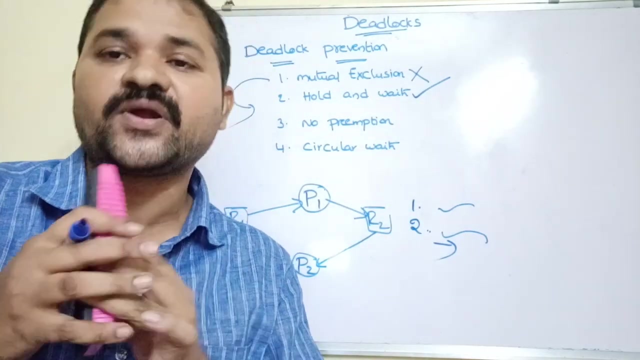 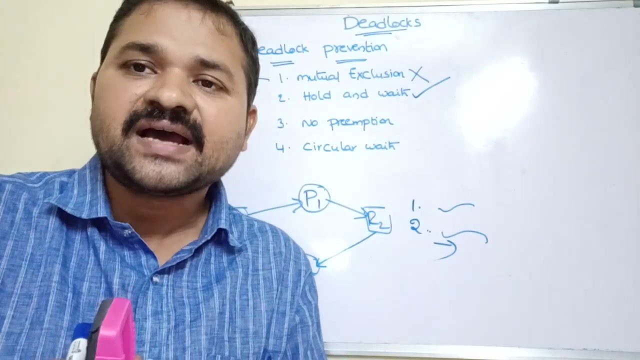 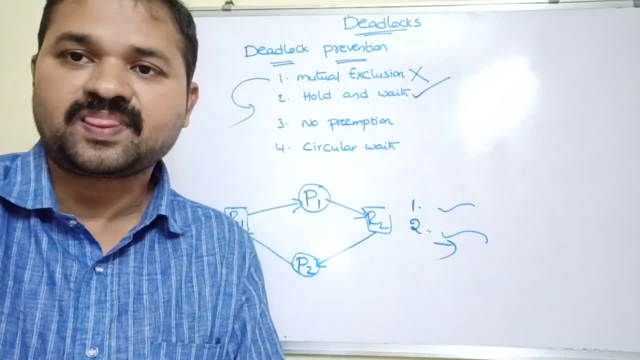 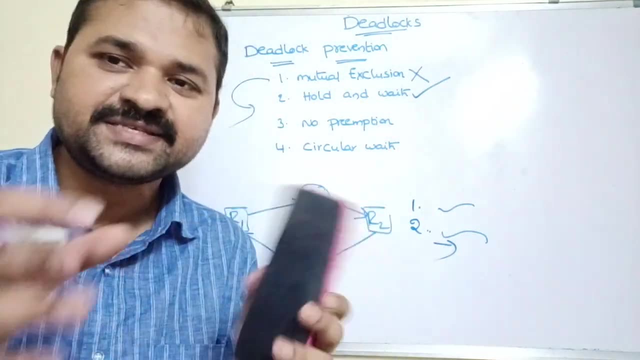 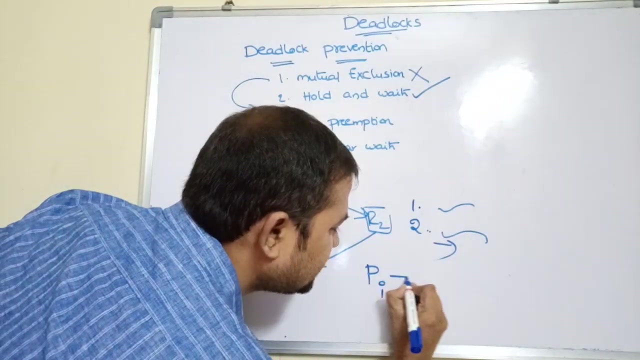 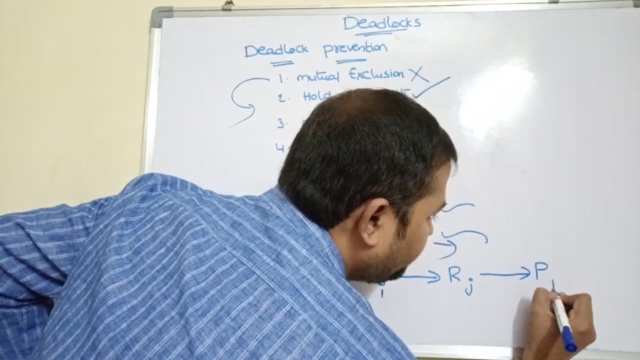 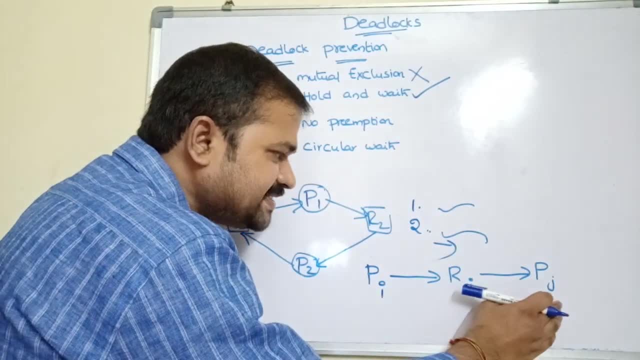 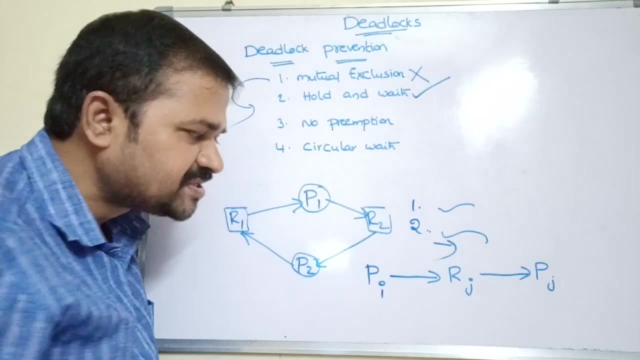 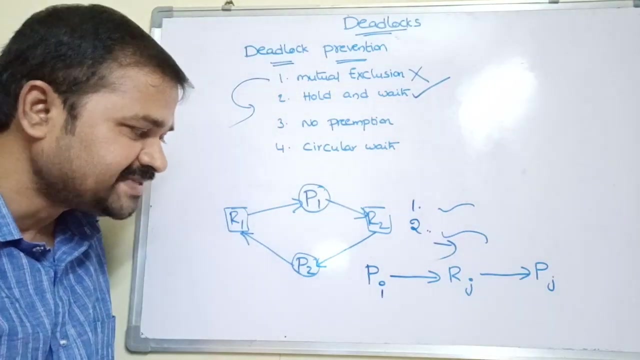 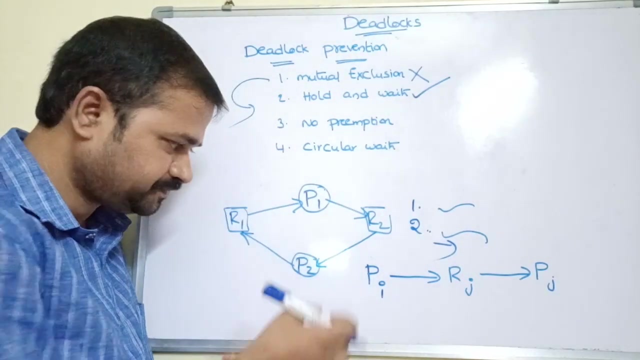 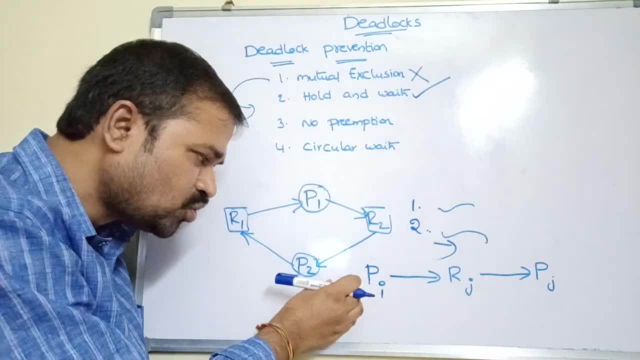 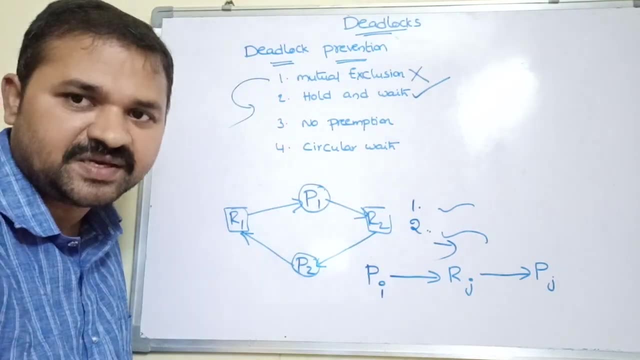 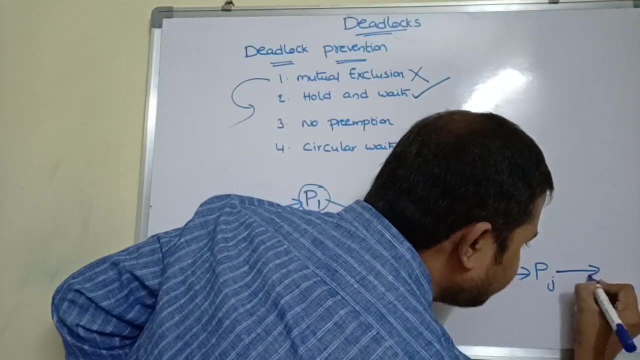 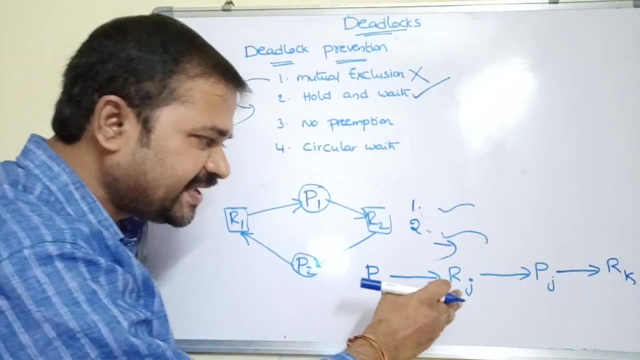 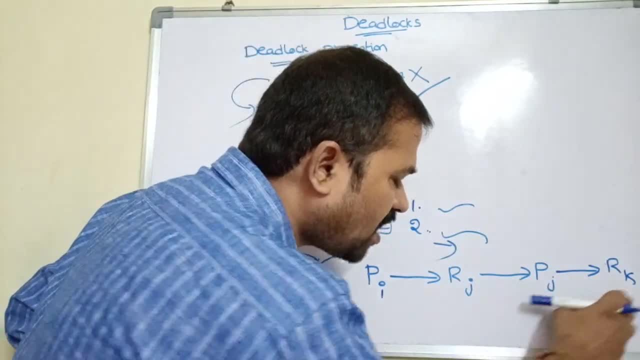 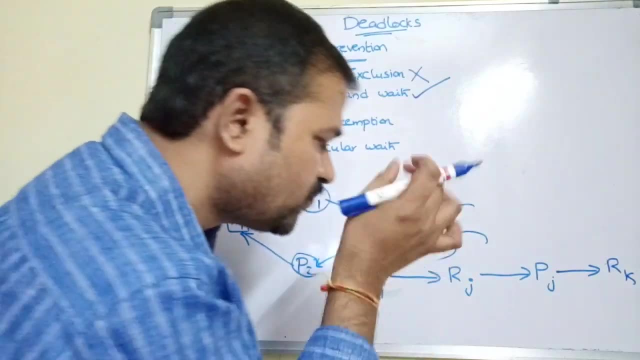 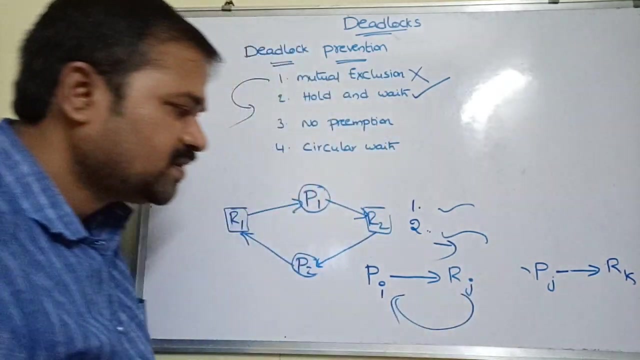 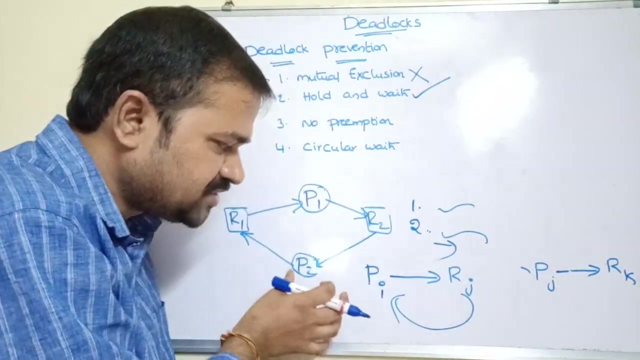 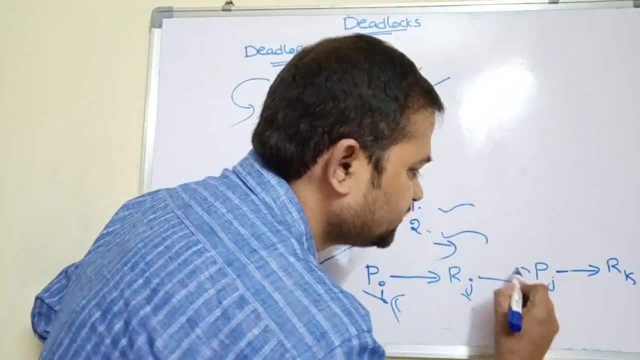 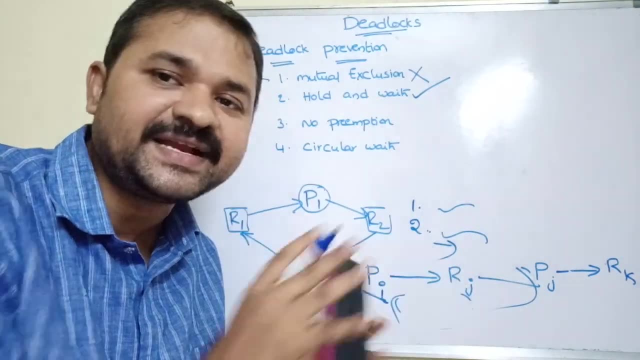 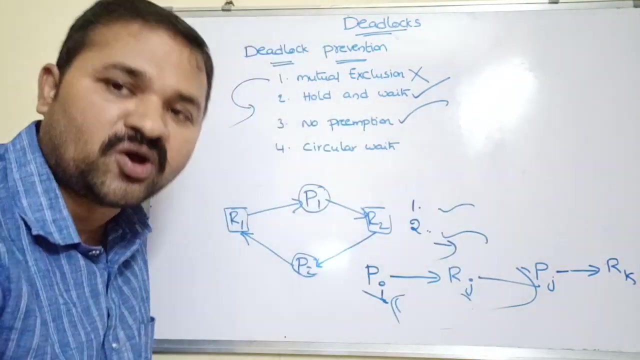 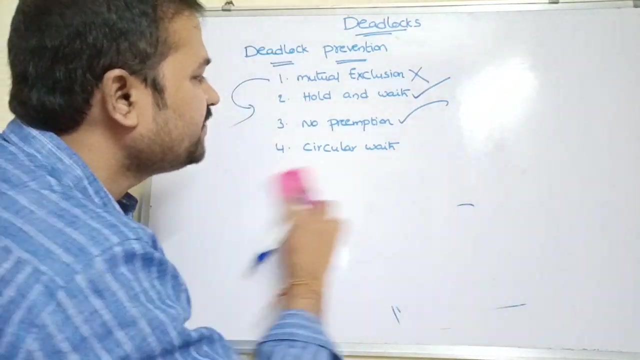 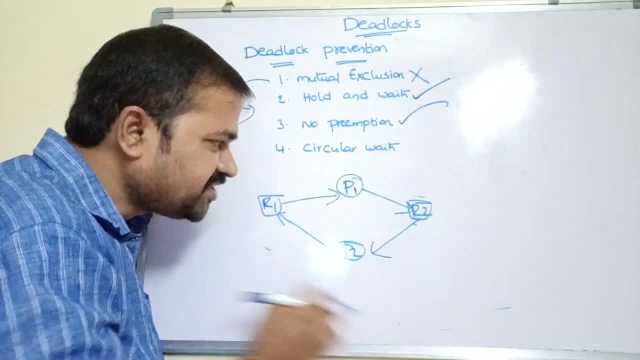 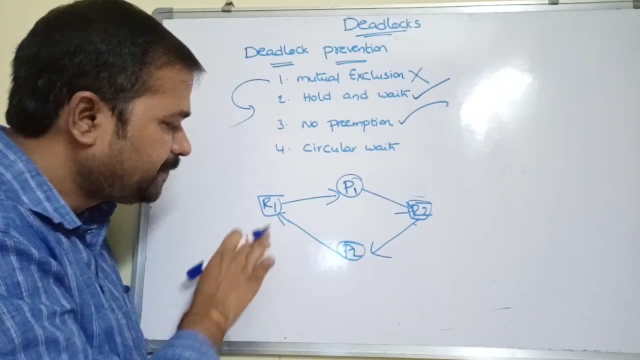 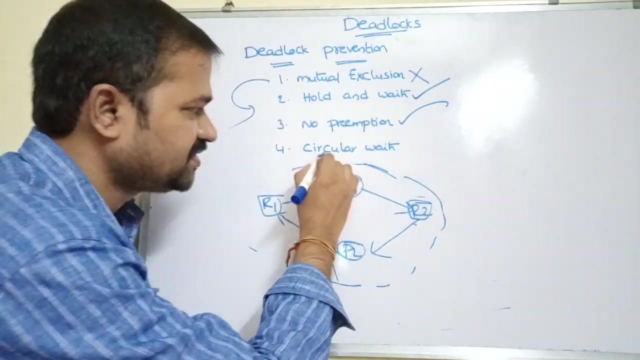 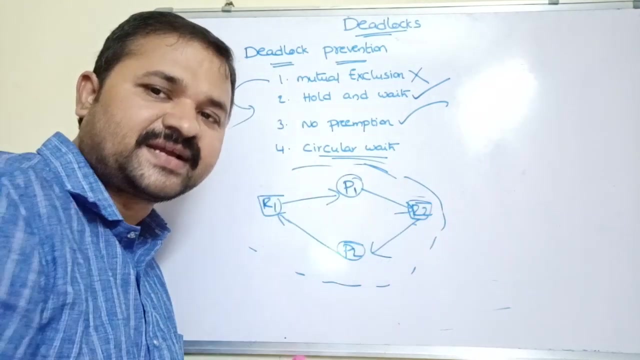 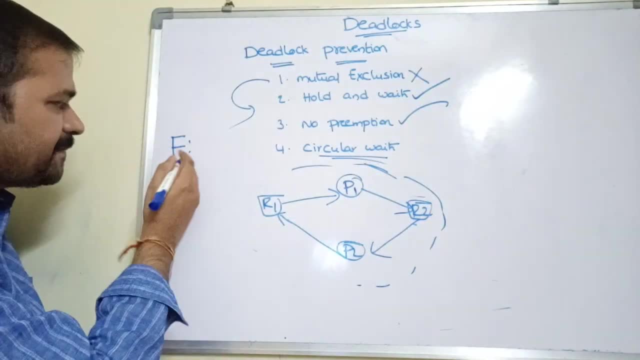 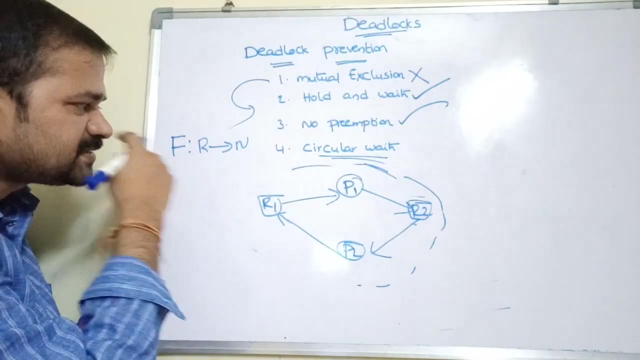 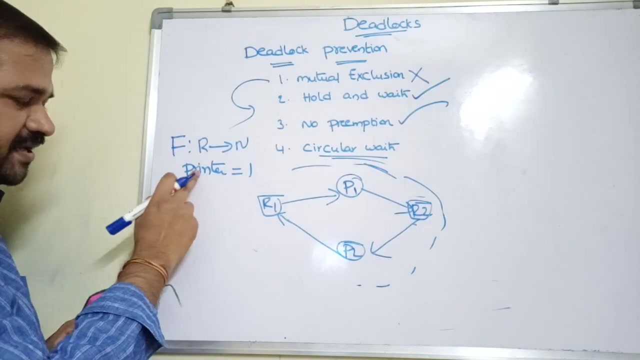 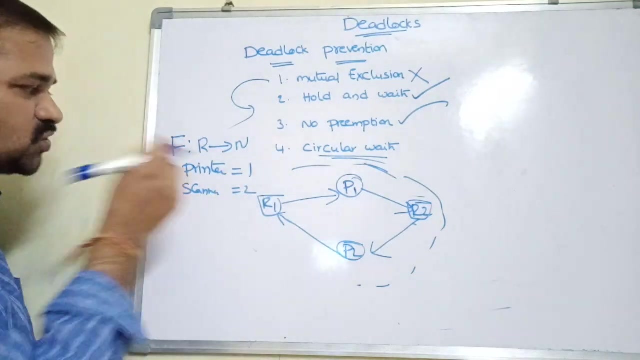 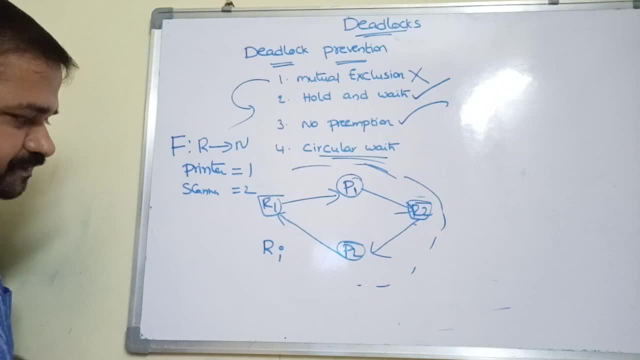 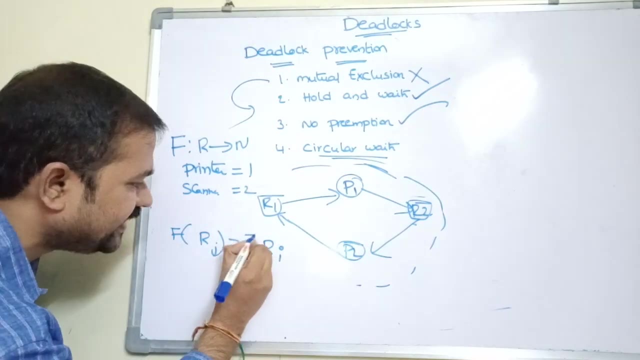 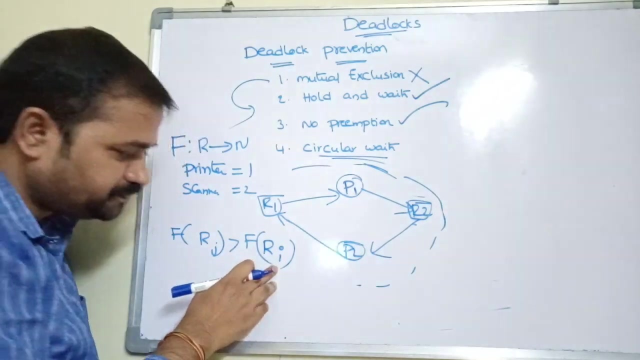 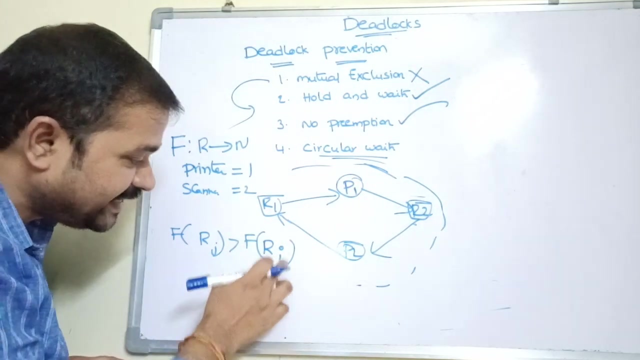 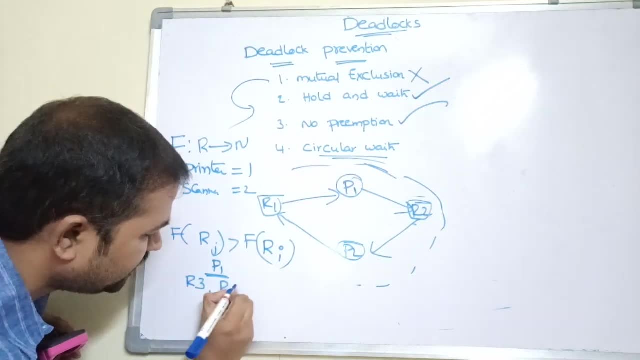 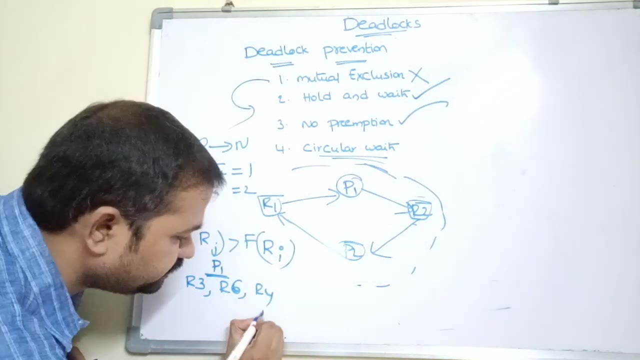 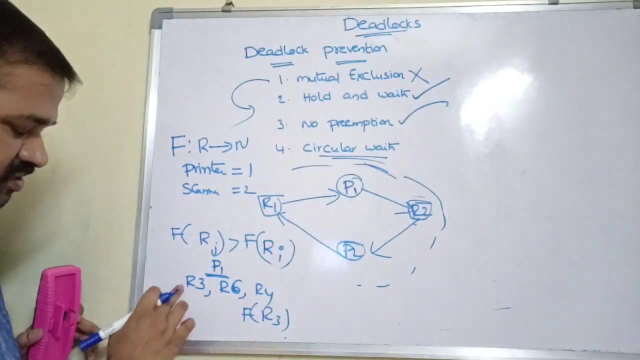 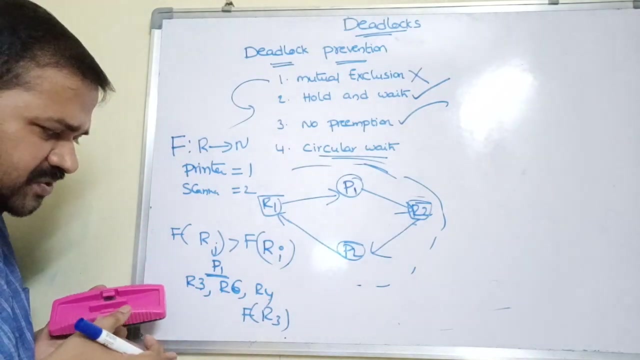